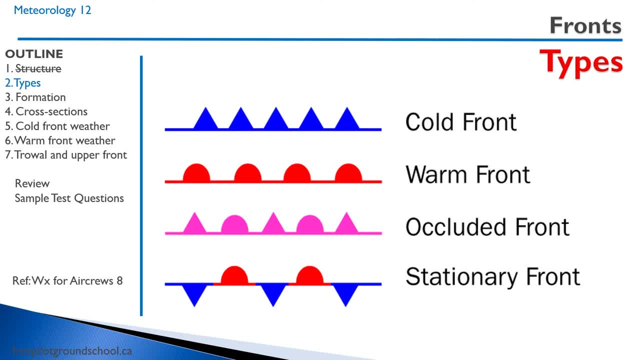 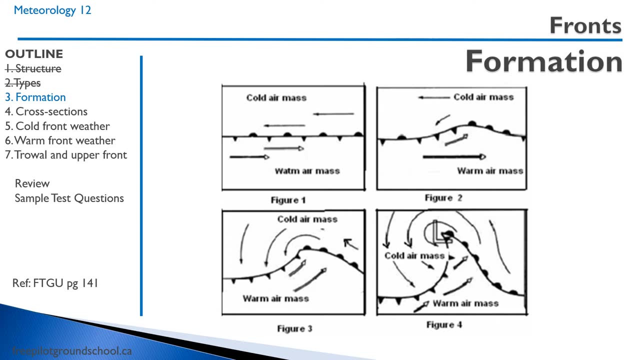 which alternates between red semicircles and blue triangles on opposite sides. We'll discuss these in a moment. Let's talk about how a front will form or a front will wave In this case. often we'll have a cold air mass beside a warm air mass. 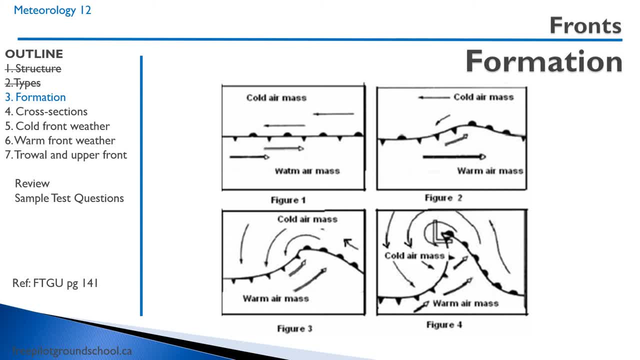 and they're moving in anti-parallel directions. Let's say the cold air is moving to the left, the warm air is moving to the right. Then eventually the warm air mass will start bulging into the cold air mass, as you can see here. This continues in figure three. 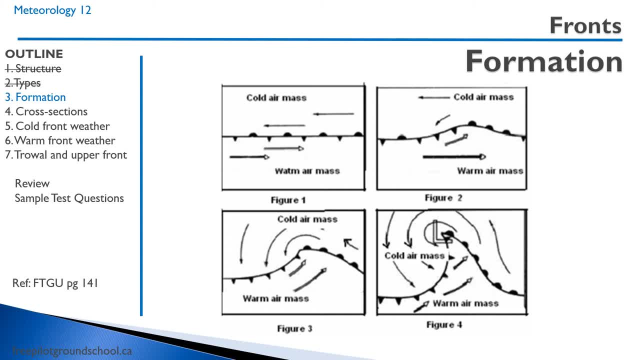 You have the warm air mass down here pressing up here, and then we have the cold air mass down here, And then this pattern continues until everything kind of catches up to one another. Then we have an occluded front which would occur up here. This is also another. 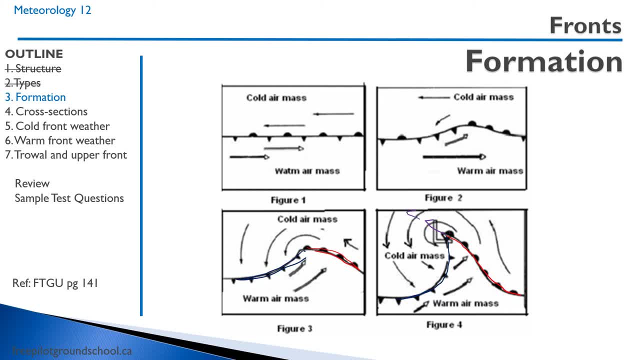 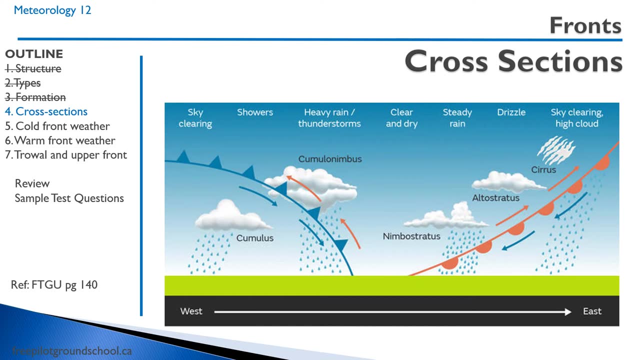 symbol for an occluded front. They catch up and then eventually the equilibrium and the air masses and moisture contents of the two are approximately the same. So here's a cross-section of a couple of fronts. The first one here is a cold front, So we would 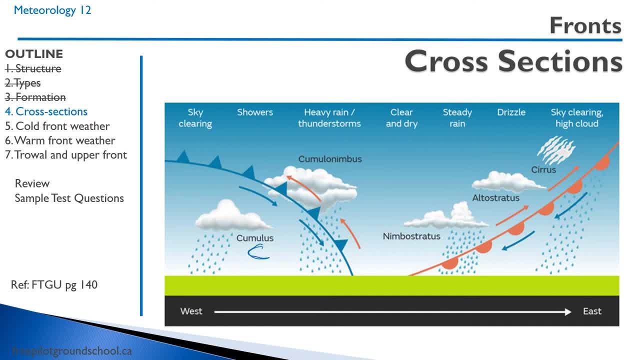 have cold air right here. So this is going to be cold advancing on warm air, or we'll just call it H for hot over here. As it forces its way underneath, it raises, pushes up this hot air, creating unstable air. 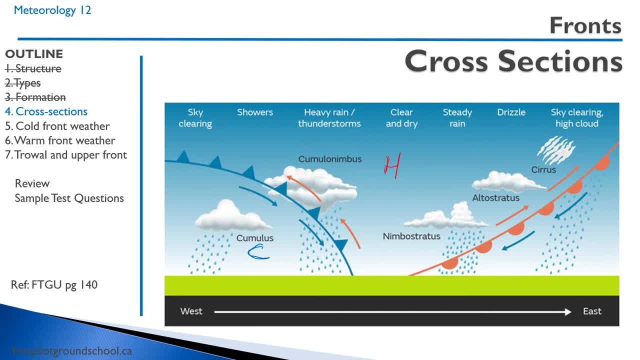 Then we look over here, This will be a warm front. A warm front will make this blue cold right here. So a warm front can either be the warm air rising up over the cold air or it can be retreating cold air. The cold air is moving this way, leaving behind this. 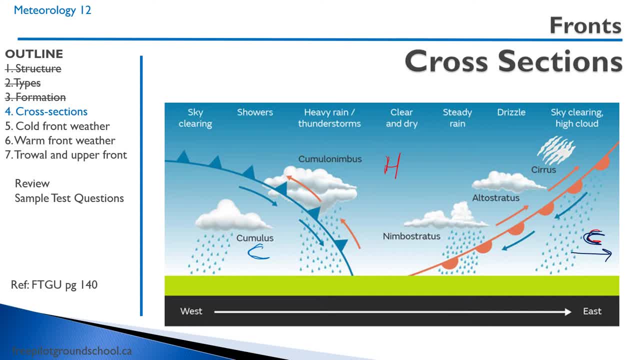 the warm air following it, Then typically in a warm front, we end up with these high clouds. When we have these high clouds, the cold air moves up with the high standards. but if you look up here, that's mainly low temperature eaten by the cold air from that. 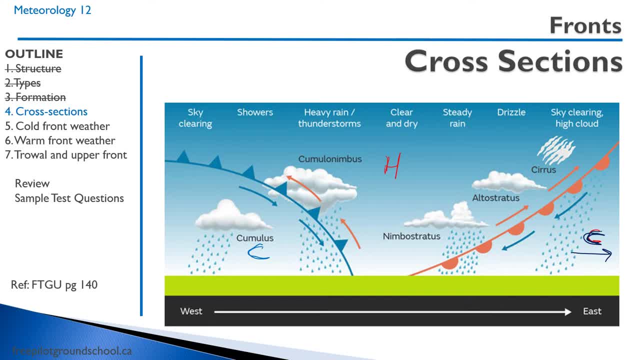 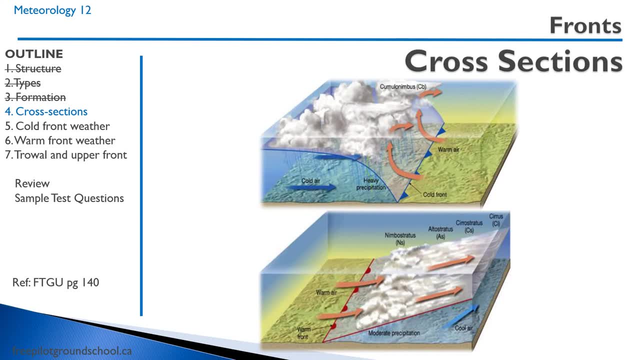 rose I just mentioned- or you could also call it the rose I just mentioned. So one thing that we have here, that's mostly stable air. these cirrus, altostratus and nimbustratus- This is kind of the characteristic warm front weather. 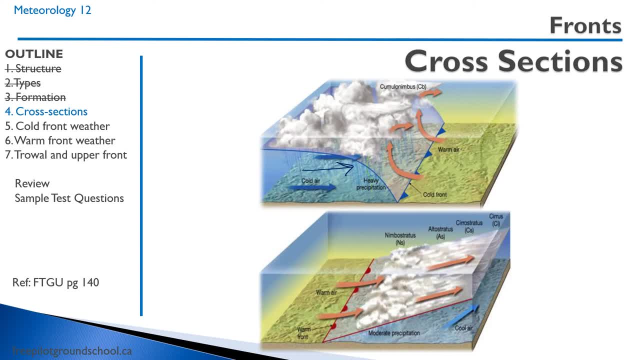 Here is a nice cross-section of uh袂 warm fronts and cold fronts. Here is the first one, the cold front. So you can see this cold air is advancing on the warm air, forcing this warm air up. We're getting unstable weather such as cumulanibus clouds. You can get thunderstorms And thenurdر у насed~. 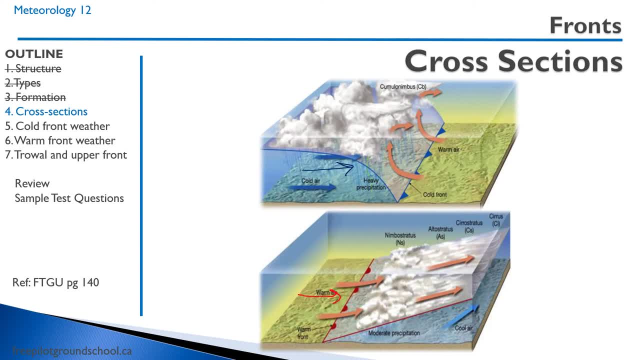 on the bottom one, we have this warm air right here. it's either advancing on the cold air or it's the cold air retreating from the warm air, and so you have this nice gentle slope. you have these cirrus, cirrus, stratus, ultra stratus, nimbus stratus type cloud formation. 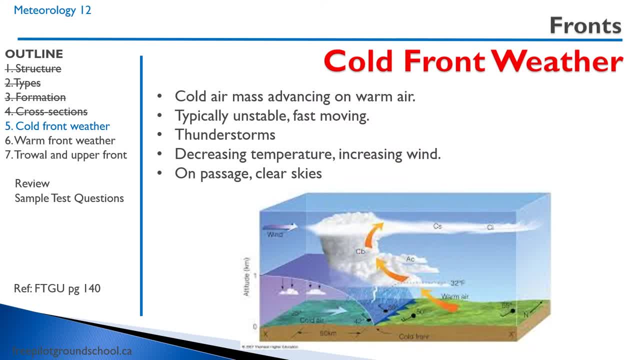 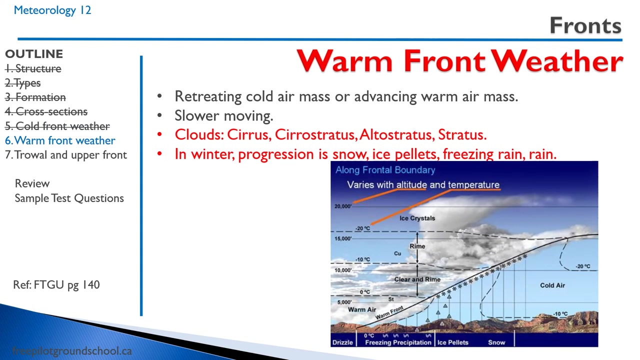 cold front weather is typically associated with unstable air, creating thunderstorms. it's fast moving. you end up with decreasing temperature and increasing wind suddenly, but when it passes you end up with clear skies because now you're completely in a cold air mass uh. by contrast, the warm front uh is considerably slower moving. and one thing you should uh pretty. 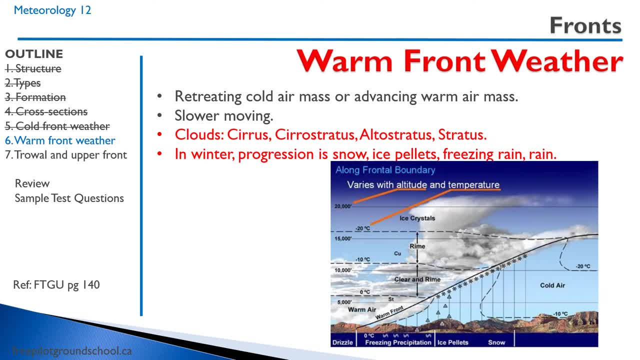 much memorize is the cloud progression, because you'll see this pretty much all the time. you start with cirrus, cirrus, stratus, ultra stratus and finally stratus, low cloud, and if you have the in the winter, we have something called a winter warm front, and it will be. 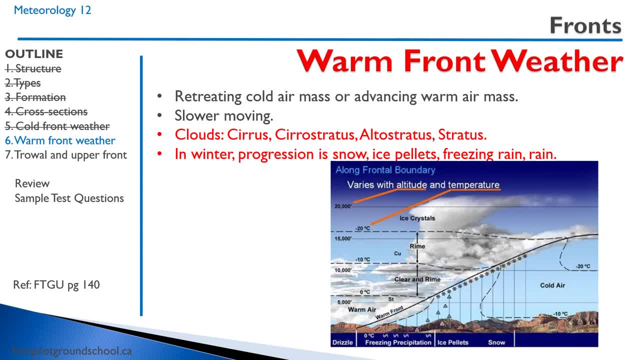 characterized by precipitation, and you'll notice this. you first start getting slow snow, then you get ice pellets, then you get freezing rain and then you get rain. so this is quite common because you have this inversion at the at first, when you get your your snow from your higher cloud. 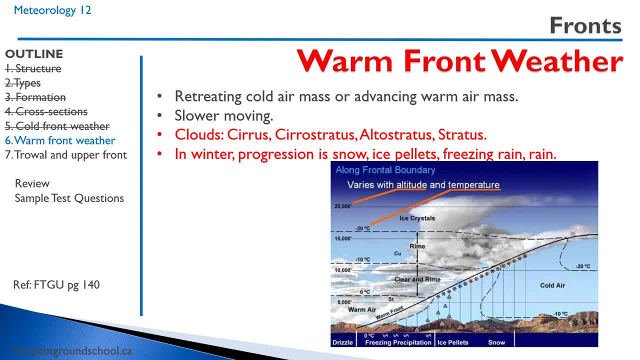 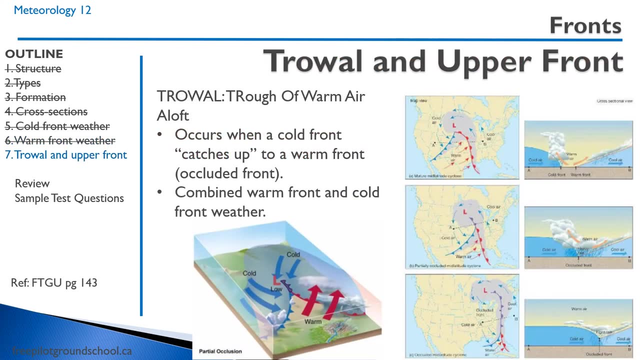 it just falls into cold air and then, as that warm front approaches, you have warm air on top, colder air down below until finally, once the front passes, you're just in warm air, causing just rain. we also have uh friends called trowels, which is a short form trough of warm air aloft. it's also called 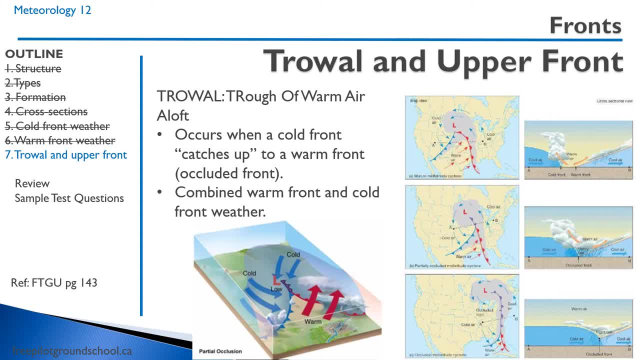 an occluded front. in the united states, canada they call it a trowel, the symbol slightly different, so i showed you earlier the symbol: uh, with an occluded front is alternating a red and blue triangle and semi-circles. And then in Canada we have what's called the trough of war and arrow loft. 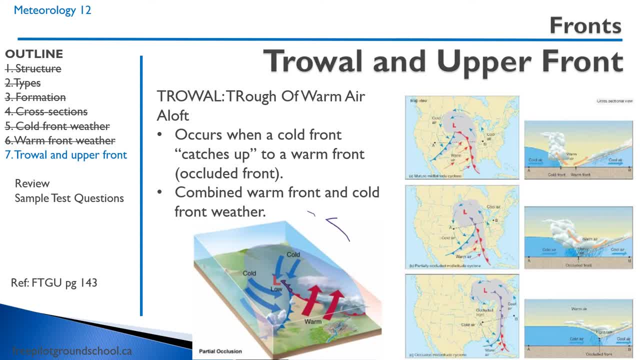 You can see this here, and it's actually magenta and they make these arrows. okay, And this occurs when you have a cold front catching up to a warm front at a certain area. So take a look on the left, We have an area. Let's just say we're right here, okay, So we just went through warm air. 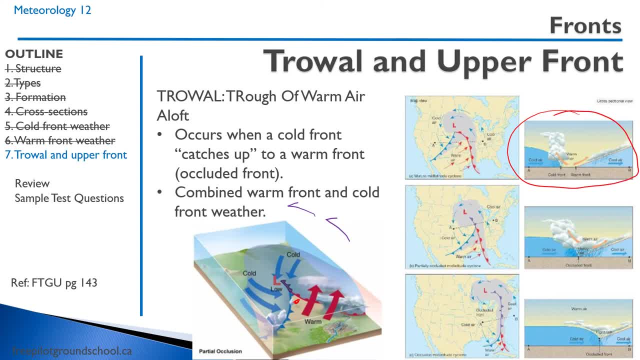 or just through a warm front. So here's the cross-section, right here, We look at it, We're sitting right here. This was the first what I said. So we just went through a warm front and now the cold front's approaching. That's what we see. However, as time goes on and let's just 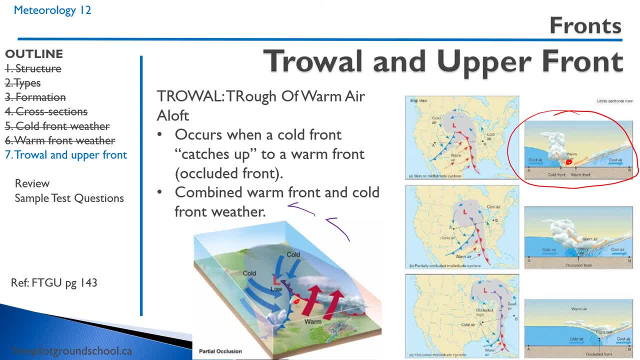 say: I'm just going to make this a different color so we can figure it out. We're going to be purple, right here. So we're right here, and this is this, right here. okay, The cold front has caught up to the warm front, okay, So now you have two different fronts and up here you have a trough. Here's the. 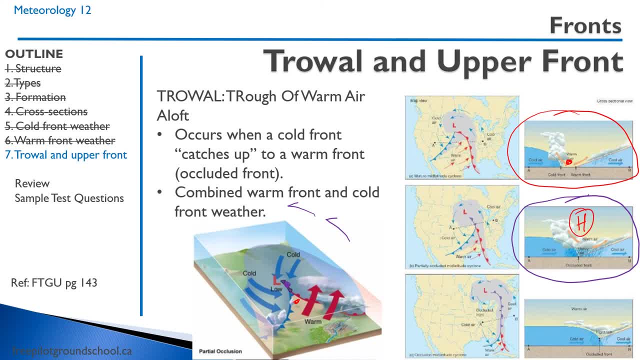 warm air, right Or hot, okay. So this is the trough of warm air. See how it kind of makes a trough up here of warm air aloft, And so you get the worst of both fronts. You end up with things like freezing, rain and thunderstorm. 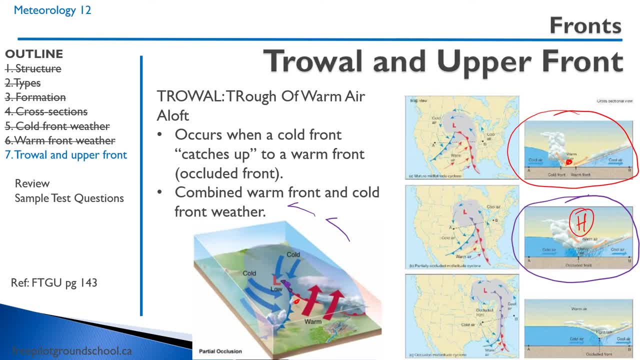 at the same time, and it's just absolutely miserable. And then, lastly, let's just say we're up here at the top and that's this right here. Now we've pretty much it's kind of equalized itself out. You have cold air and cool air, and it's considerably higher. The weather has kind of. 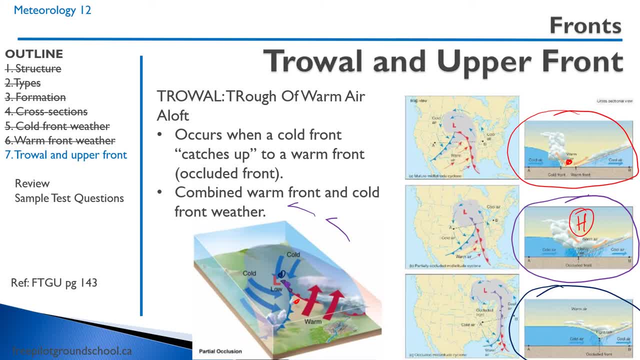 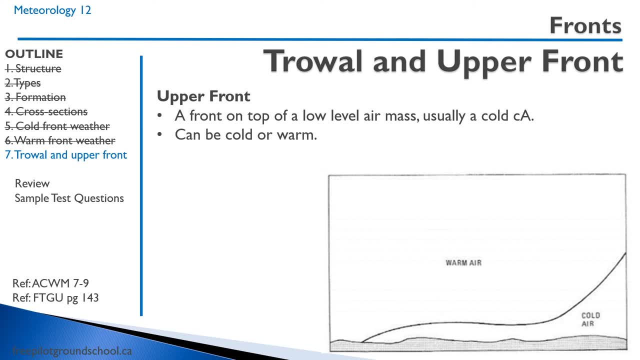 come up at this point and we just the warm air is above. We can also have upper fronts, which is when you have a front on top of a low-level air mass. So here is a picture or diagram: cold air and you see this upper front right here, This cold, it's sitting the front's right here, but it's. 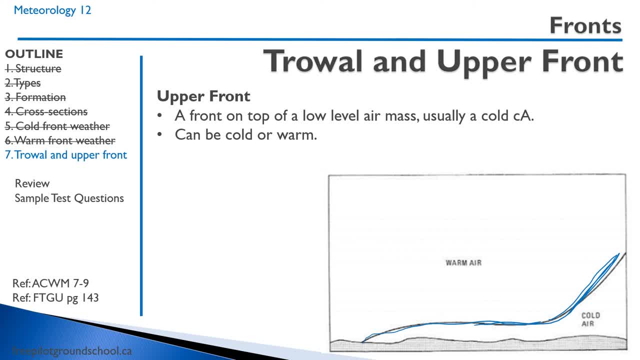 sitting on top of this cold air mass, So you it can be cold or warm, You just end up getting frontal weather, but the cold air it's. you know it's not as cold as you think it's going to be, but it's. 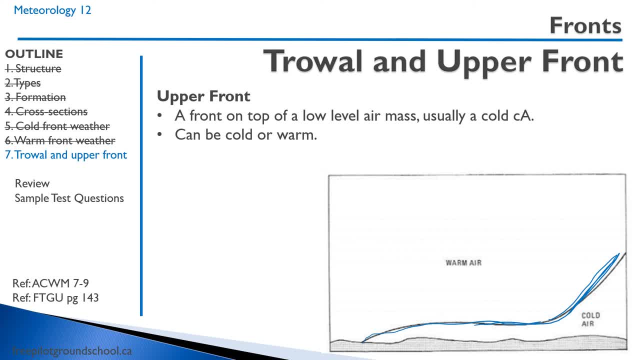 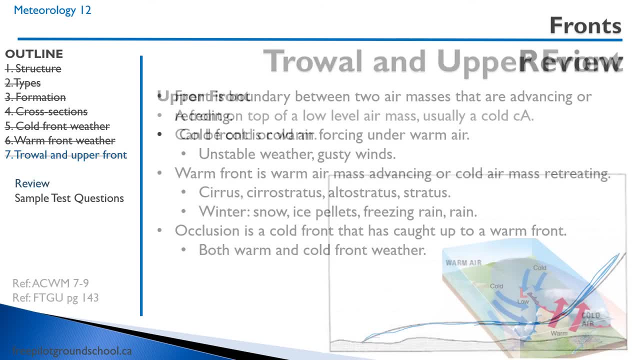 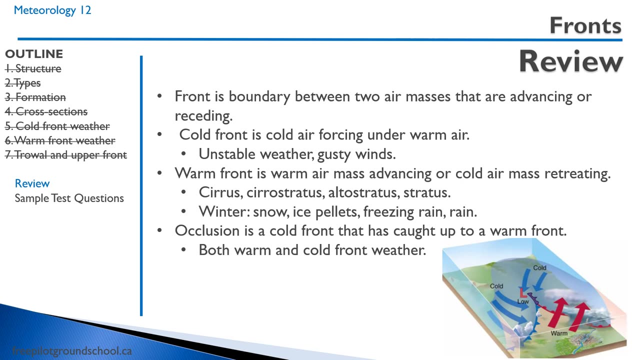 below. So this might still be, let's say, a warm front, but it's still freezing cold for a while until this bottom air mass clears out. A front is the boundary between two air masses that are advancing or receding. A cold front is cold air forcing itself under the warm air It's associated. 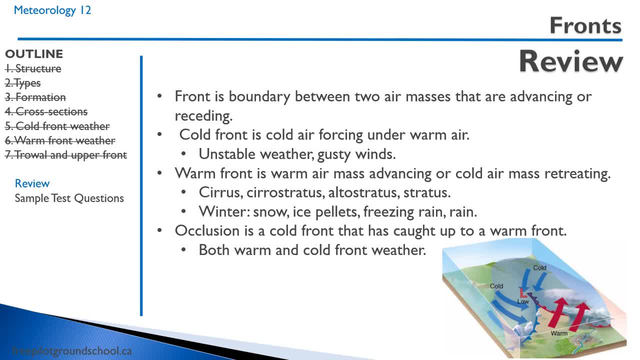 with unstable weather and gusty winds. A warm front is a warm air mass advancing or a cold air mass retreating. The weather associated the clouds are cirrus, cirrostratus, altus and stratus. In the winter we can get these winter warm fronts where we get snow ice pellets. 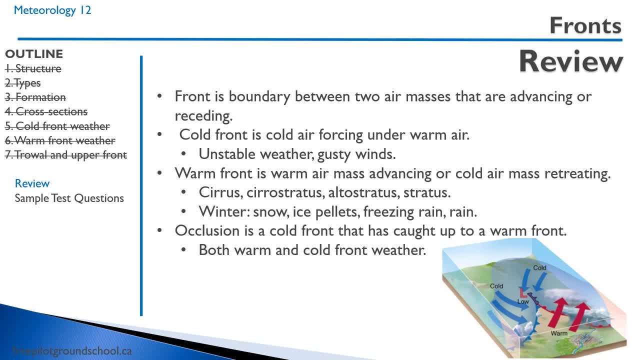 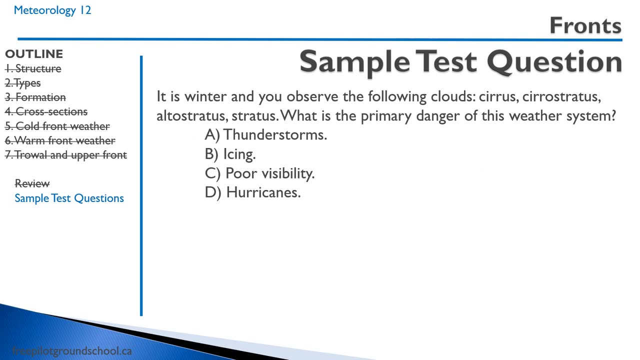 freezing rain and then rain. An inclusion or a trowel is a cold front that is caught up to a warm front. You will end up with both warm front and cold front weather. It is winter and you observe the following clouds: cirrus, cirrostratus, altustratus stratus. What is the primary danger? 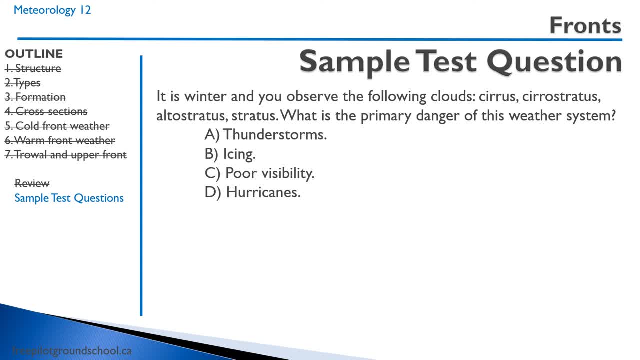 of this weather system. So remember what kind of front is associated with these clouds. Well, that would be a warm front. And what kind of precipitation in the winter will we get from a warm front? Well, we'll get things like ice pellets and freezing rain. So icing is going to be a big, big consideration. That's going. 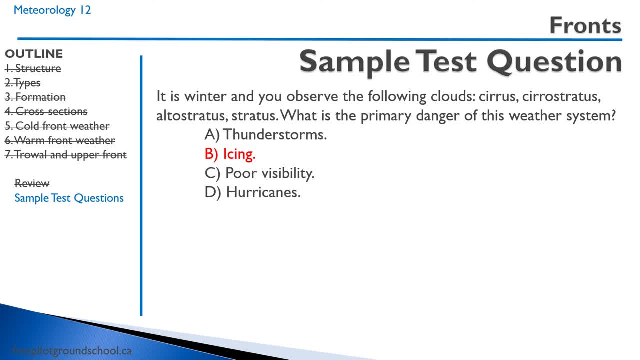 to be the most dangerous thing. It's not going to be thunderstorms. We're not going to see thunderstorms in a winter warm front And, yeah, you might get core visitability, but that's not nearly as bad as the icing. And then hurricanes- no, we don't really deal with that, It's not. 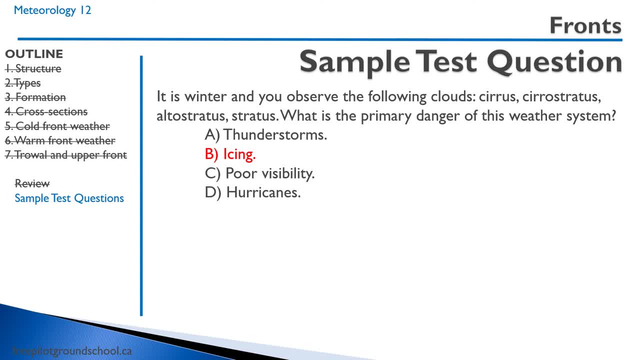 really typical of our weather systems in Canada, although we do have a lot of weather systems in Canada. We can get hurricanes in the maritime regions. The cold front is primarily associated with what type of weather. So remember a cold front we're going to have, it's the cold air. 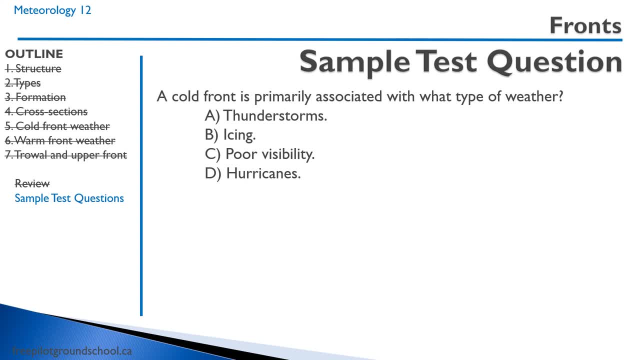 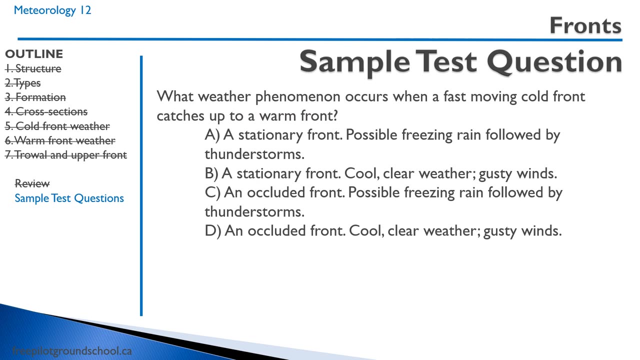 forcing its way under the warm air, pushing warm moist air up, So it's going to be unstable. You're going to end up with thunderstorms, with cold fronts, And the faster that cold front moves, the bigger the thunderstorms will be. What weather phenomenon occurs when a fast moving cold front? 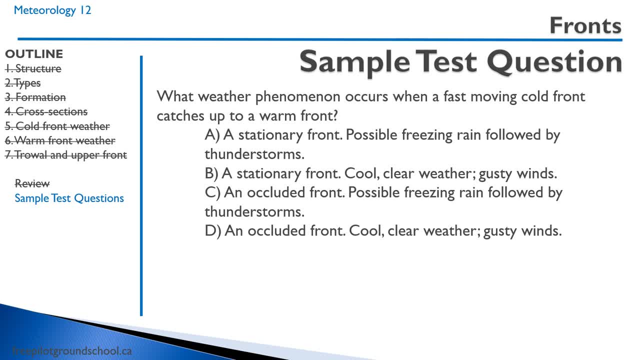 catches up to a warm front, Well, that's going to be a cold front. So it's going to be a cold front. So remember, when you have a cold front catching up to a warm front, we call that an occluded front. 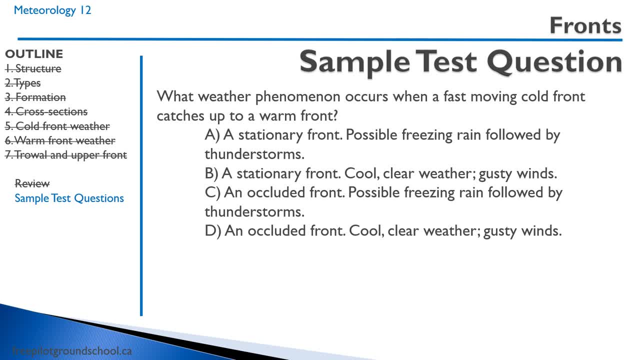 which causes a trough warm air aloft. So you get both cold front and warm front weather. So you start with possible freezing rain. Let's say we're in the winter, So it's a possibility, but then we follow it up with thunderstorms, So kind of the worst of both worlds. That concludes this lesson. on fronts. Thanks for joining me And we'll see you at our next lesson.